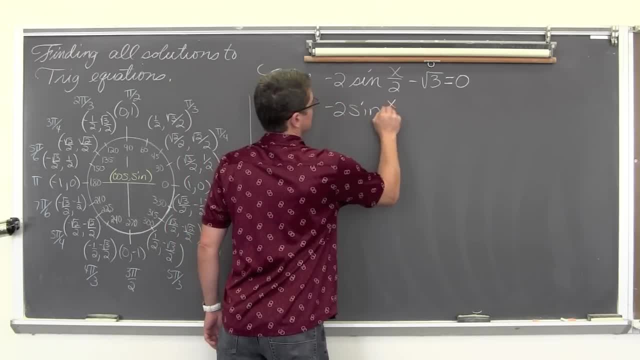 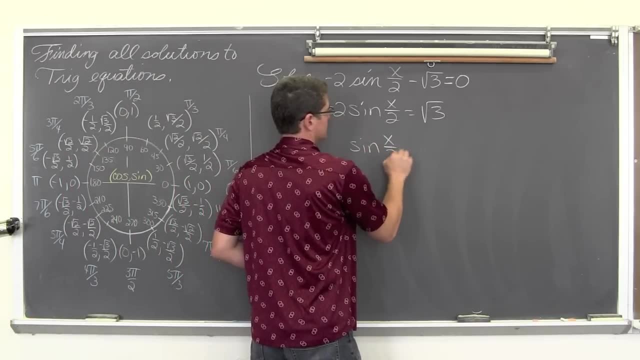 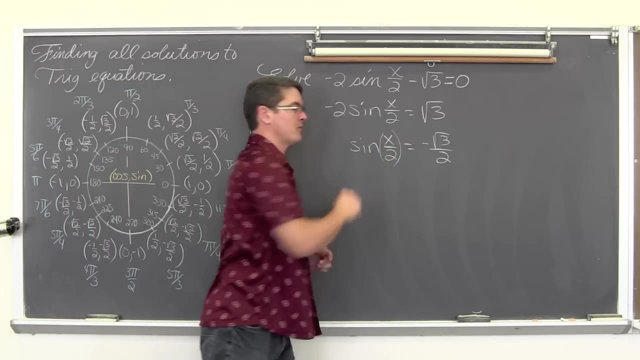 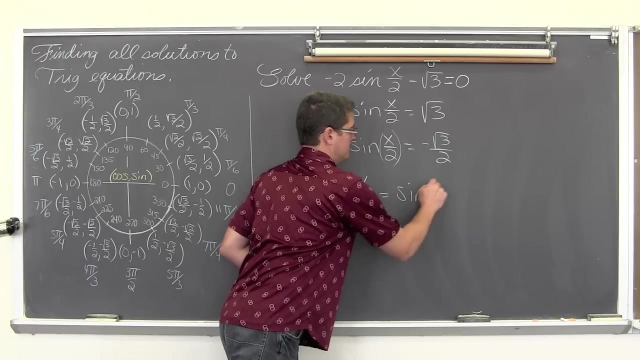 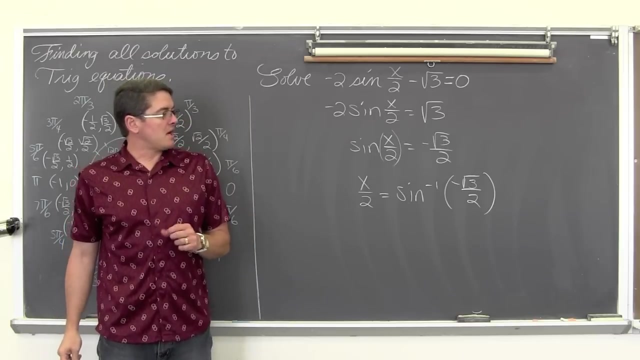 to both sides. We are going to divide both sides by negative two. We are going to get the sine function away from our angle. Remember it is an angle measure we put into trig functions. by doing inverse sine We get x over two equals the inverse sine of negative square root of three. 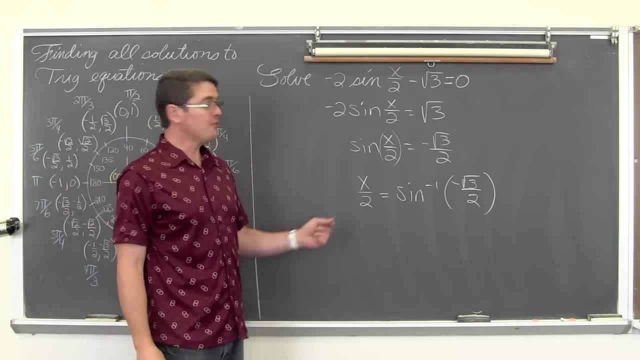 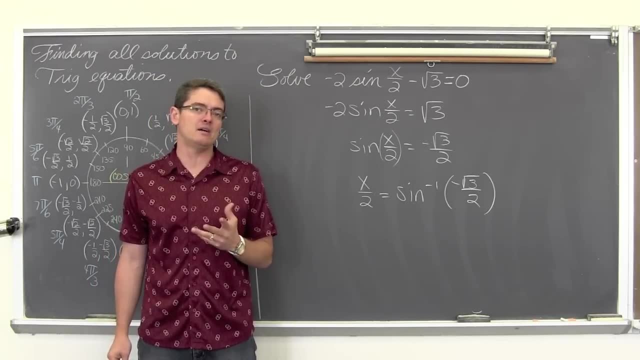 times x BAM. Mr Tarrou, In this video we are going to take a look at solving trig equations again. Now, if we were looking for answers that we had restricted answers between zero and two pi, this equation would not have a solution, Because when you have a half angle in your 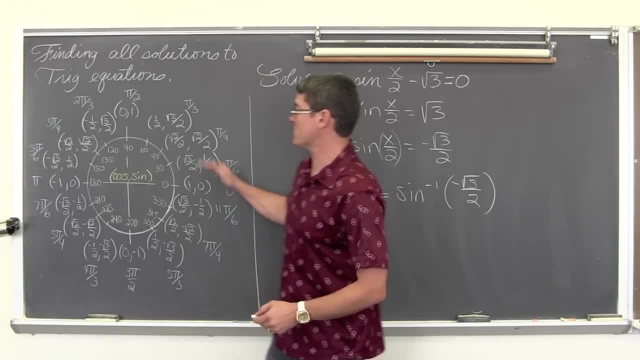 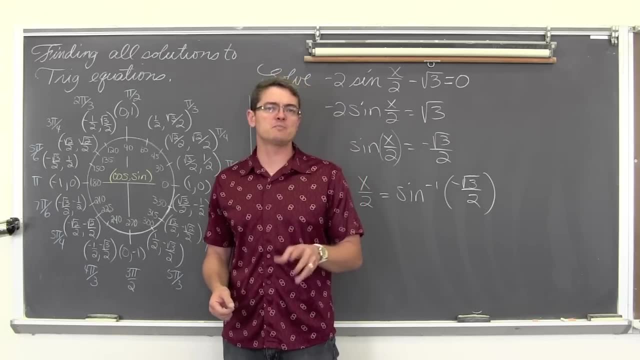 trig function. if you have a half angle when you talk about your unit circle, you are only going to go half way around it, So that when you multiply by two you will have all your angle measures be between zero and two, pi over three, sixty if you are doing degrees. 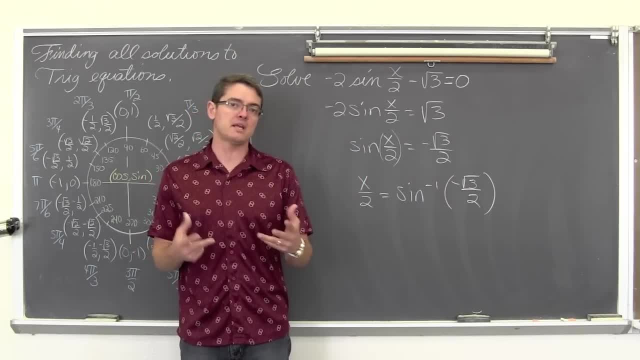 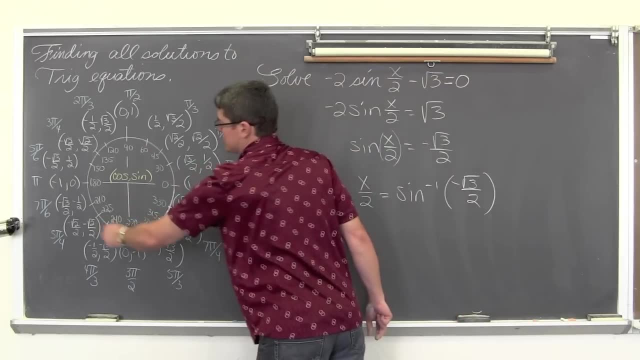 So if we had a restriction on our values that we are allowed to give as answers, this would actually have no solution. But since we don't- and we are looking for all possible solutions- we are going to go around this unit circle until we find those angle measures. 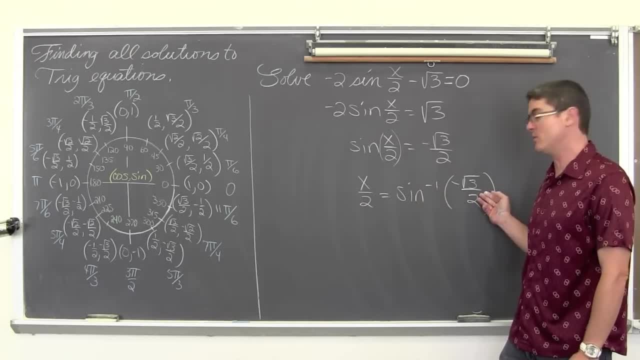 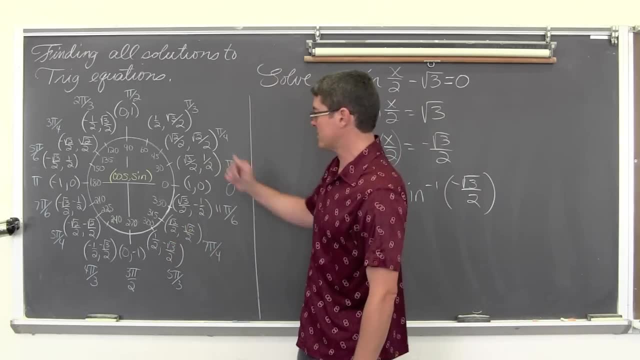 That is what you get from an inverse trig function, Those angle measures that give you a sine value which is equal to negative square root of three over two. The sine function is y over r, so it is the y values on the unit circle. We have one here at four pi over. 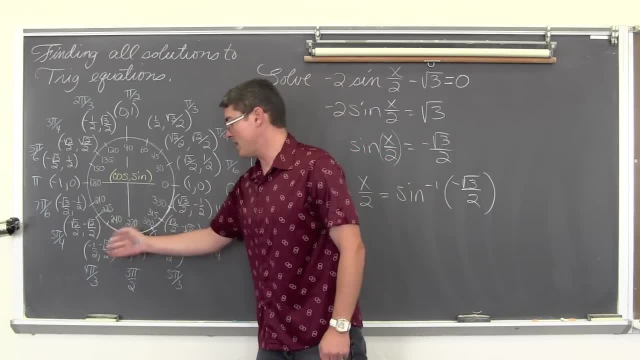 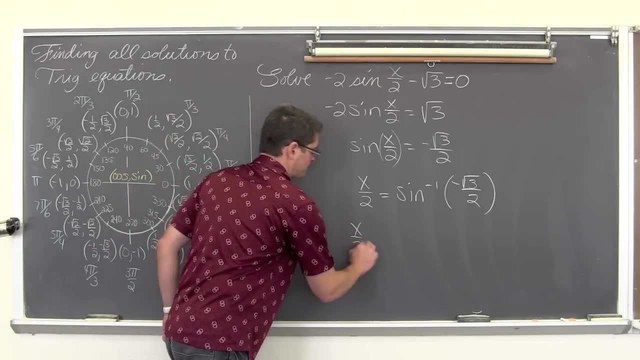 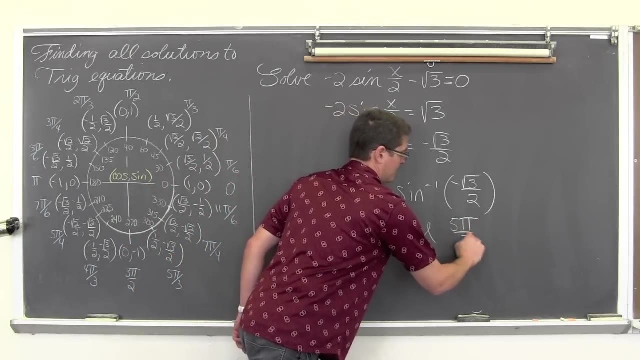 three and five pi over three. BAM, Mr Tarrou, In this unit circle we have four pi over three and five pi over three, Our angles in quadrant three and four, where the sine function is indeed going to give you a negative ratio. So x over two is equal to four pi over three and five pi over three. 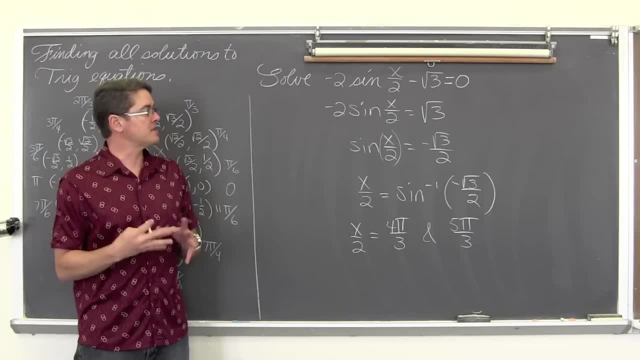 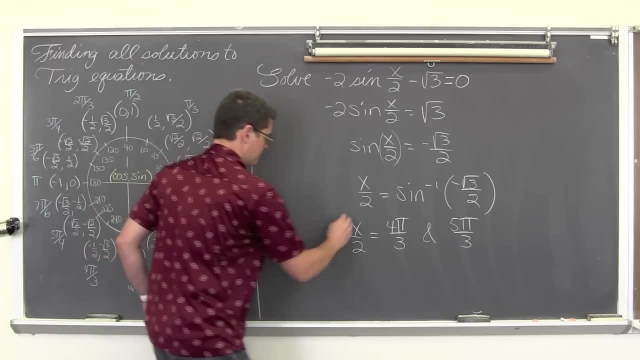 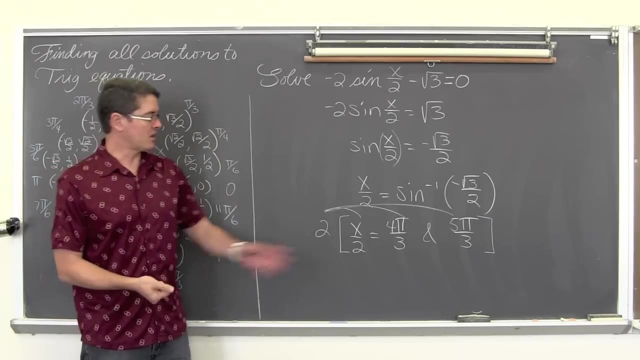 But we weren't asked to solve for the angle measure that is inside the sine function of x over two. We are trying to solve for x, So we are going to multiply everything by two to get rid of this division of two. Just put it all the way through that I guess you could argue. I have really two equations. 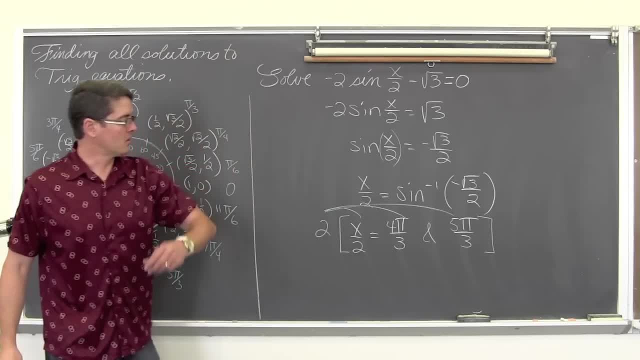 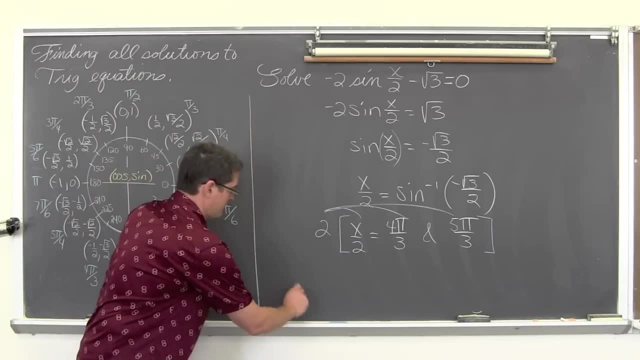 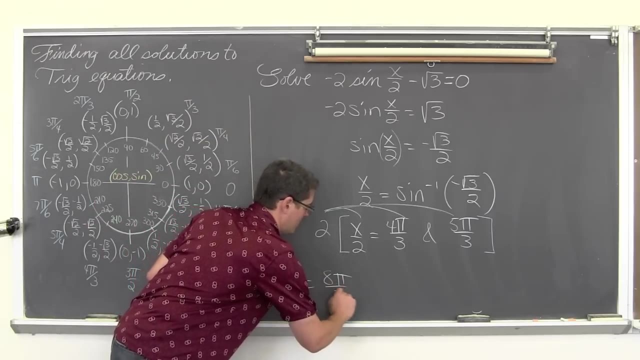 here, because x over two equals four thirds pi and x over two equals five thirds pi. But anyway, we are going to multiply everything by two and get. x is equal to two times four, is eight over three, So eight pi over three and two times five pi over three, which. 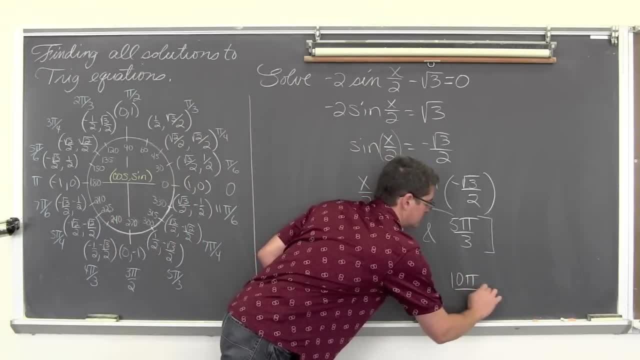 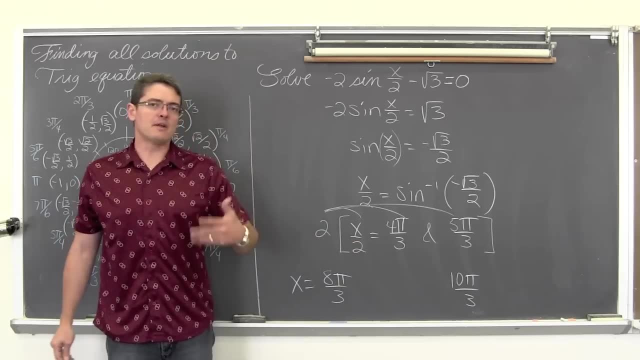 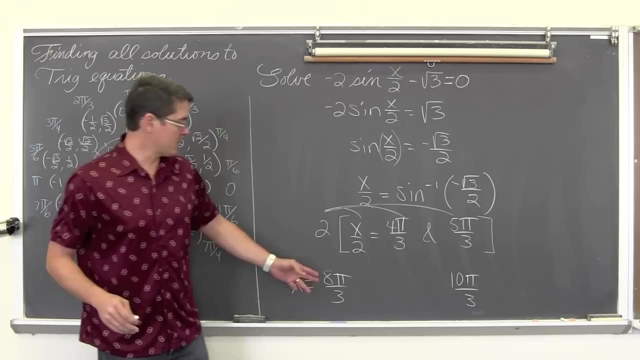 is ten pi over three. Leave in some space, because I know I am going to have to add something to these answers, to express that I am looking for all possible answers, not just these two specific angle measures. Please note again that these are outside the standard restricted values for. 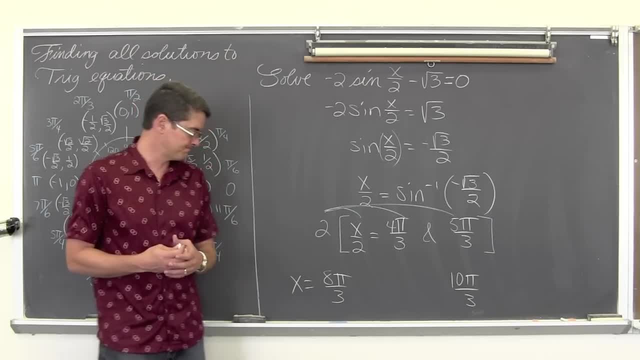 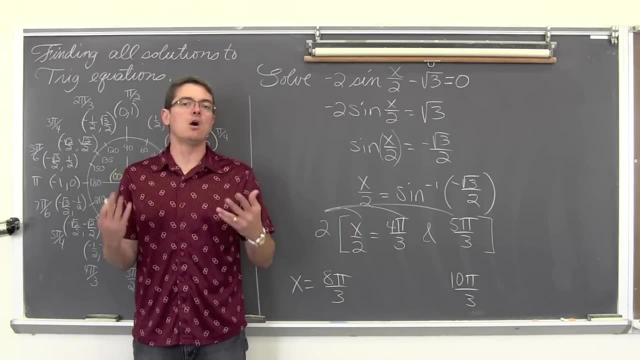 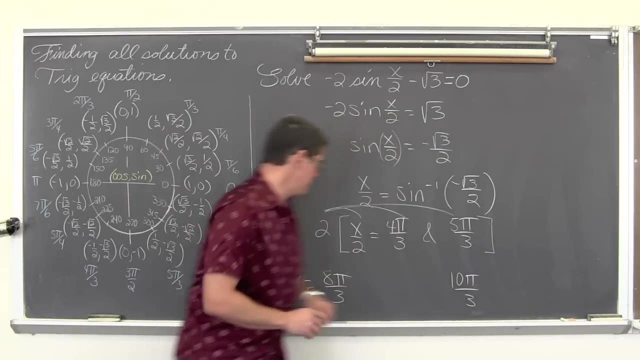 your answers with these questions of zero to two, pi over zero and three sixty. So what do I need to do? What do I need to add to these expressions to show that I am accepting all possible angles? Well, I need to do a plus. let's see where is another color here. I need to add in: 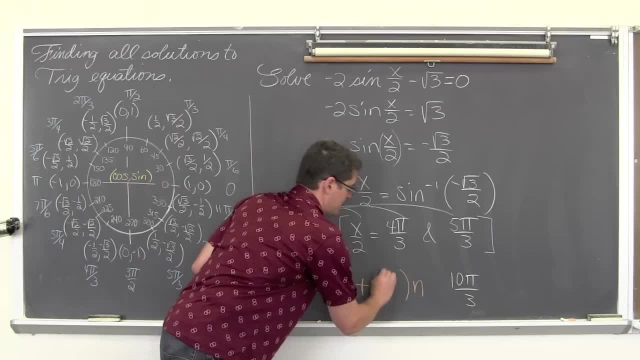 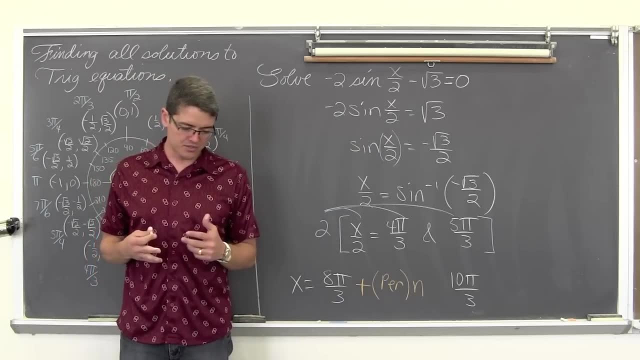 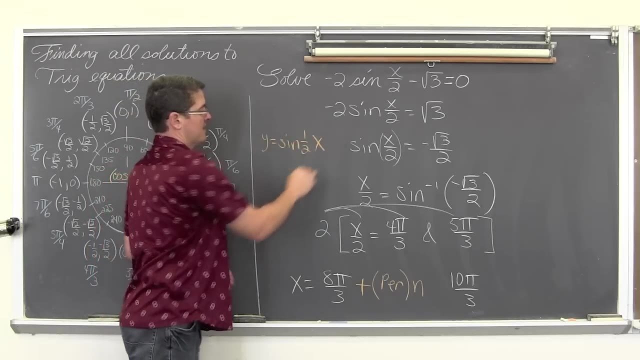 the period of the function times n. Well, what is the period when you remember graphing like y equals sine of x over two? if you were graphing this, you would be graphing: y equals the sine of one half x. That is probably how I would look at it in the section general. 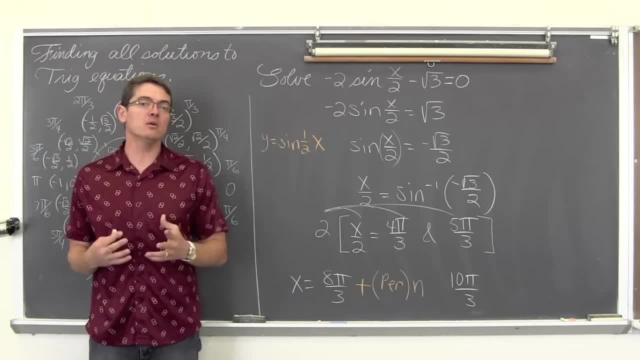 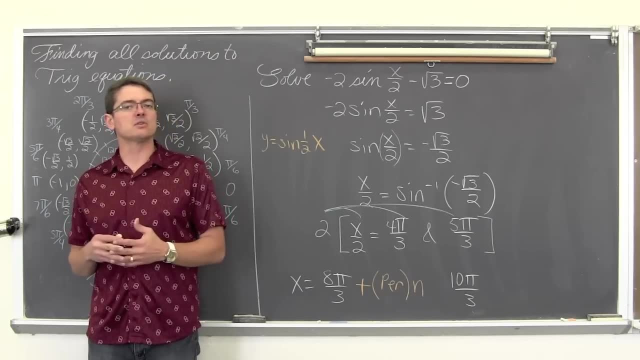 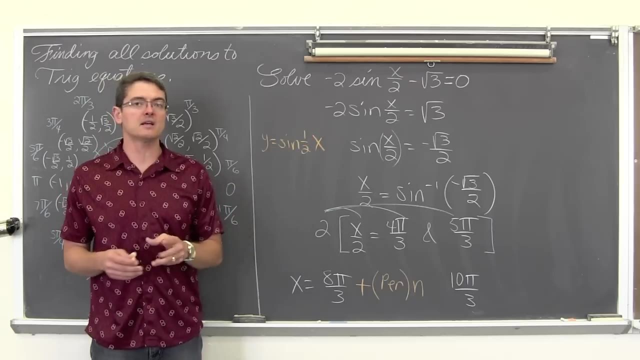 This is the value of b Period. for sine, cosine, secant and cosecant is two pi over b. For tangent and cotangent it is only pi. So the period of this trig function of sine of x over two or the sine of one half x is two pi divided by one half The period. let 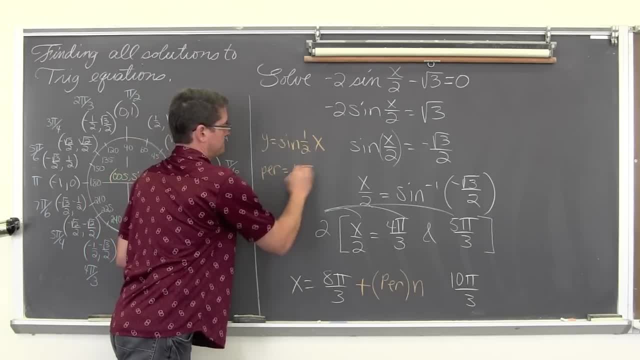 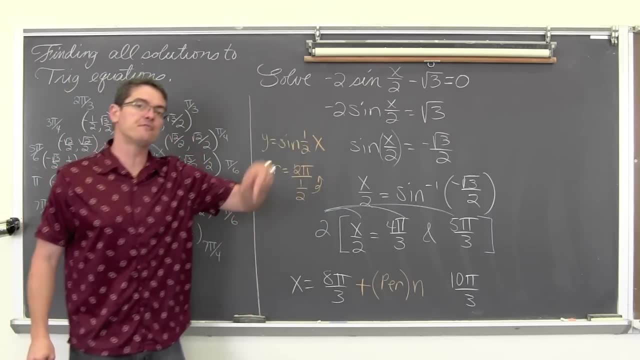 me just write it. I was going to verbally say it, but let me write it out: Two pi over three is equal to taking the one half that is in the denominator and flipping it up. So it is two pi divided. excuse me, it is two pi multiplied by the denominator, The. 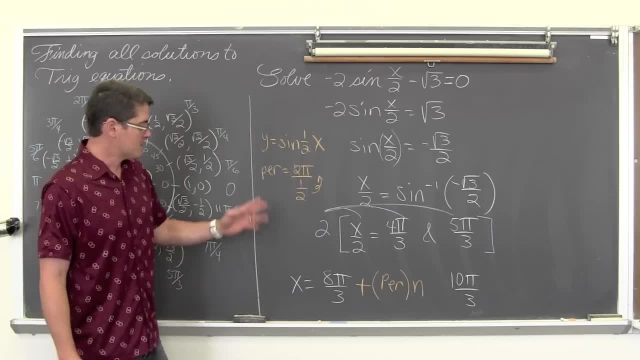 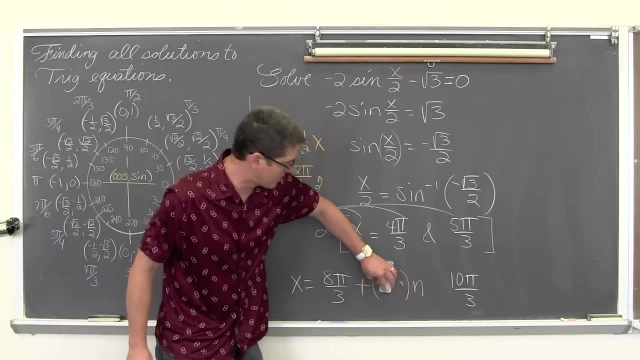 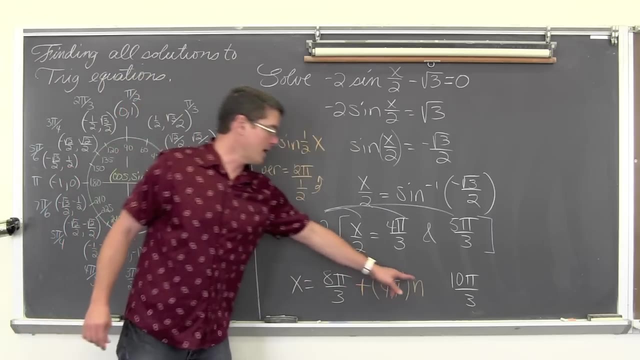 one half flipped up, So the period is actually going to be four pi. So we are going to start listing all of our possible solutions by taking eight pi over three and saying that we are going to allow it to be added by four pi. the period of this trig function n- N is. 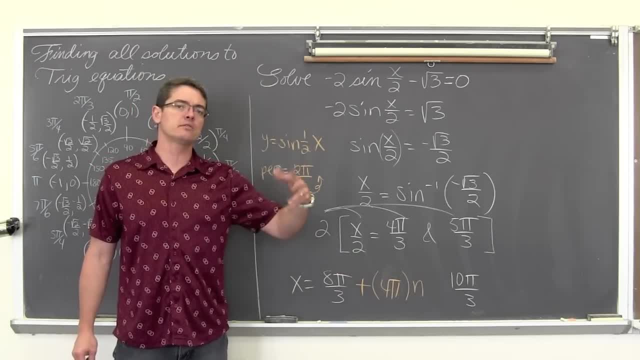 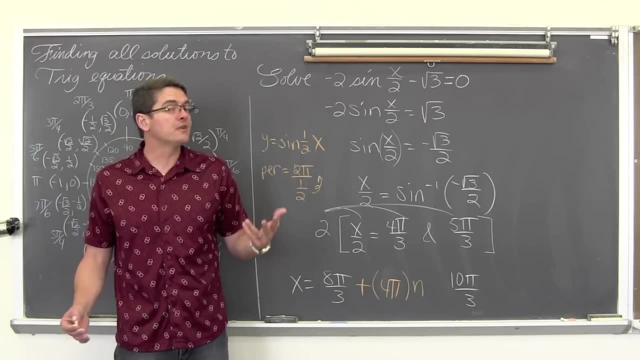 an integer n can be like negative, two, negative one, zero, one, two, three, four, five. It allows any full rotation of this period and we are going to get more and more and more and an infinite number of angle measures that will satisfy this equation And do the same thing. 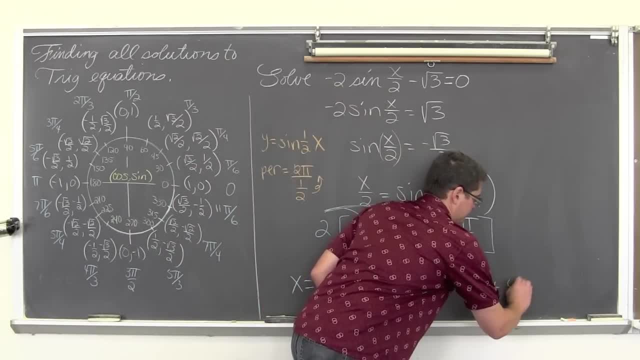 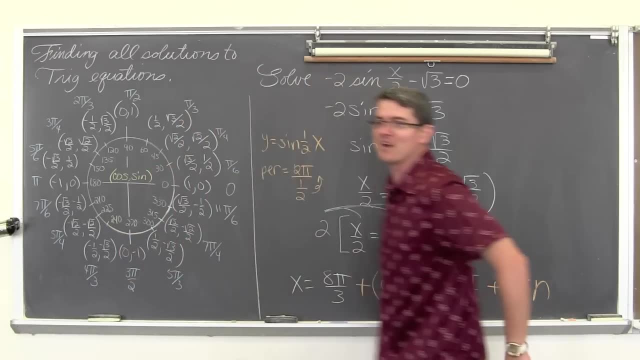 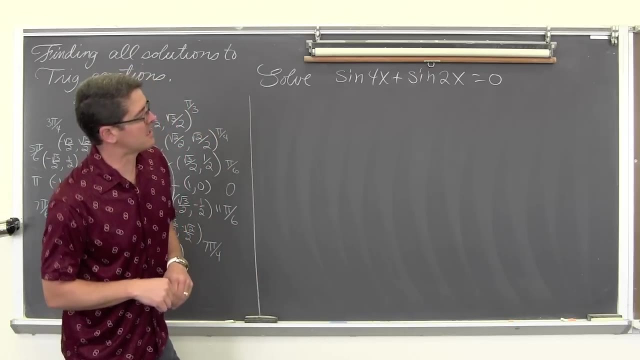 with 10pi over 3. Add that by the period of the function And then multiply it by n again, where n is an integer. So that is example one. I have one more coming WHOO. For our last example, we have the sine of 4x plus the sine of 2x, equals zero. Now it looks. 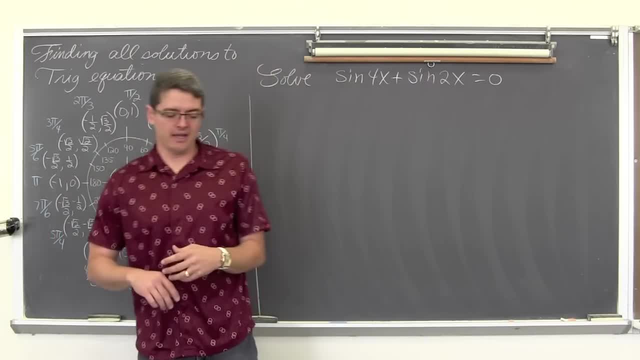 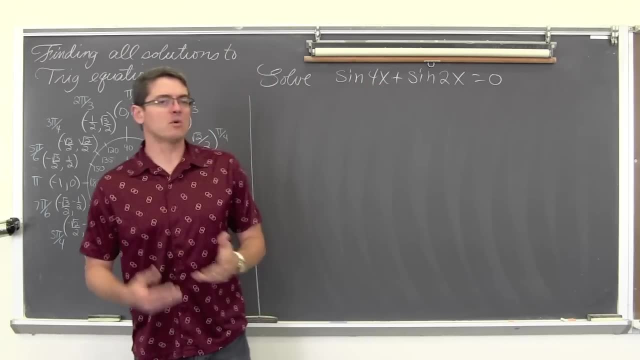 like we should be able to solve this. We have the same trig function and it should just be a little factoring to get done, But we have an angle of 4x and we have an angle of 2x. That might as well be a sine and a cosine function- This normally. this is basically. 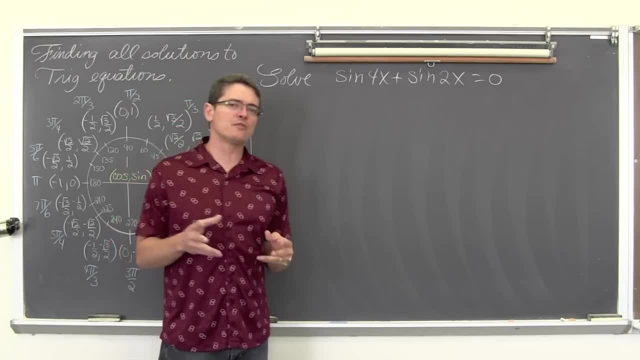 kind of the same thing. This is basically the same thing. This is basically the same thing. It is kind of like having two variables in the same equation. You can't solve for two variables when there is only one equation, unless you happen to be really, really lucky. 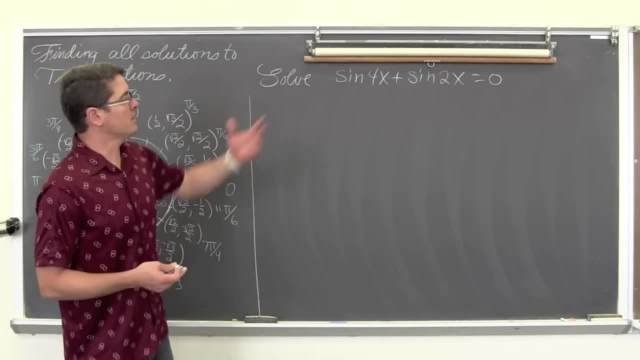 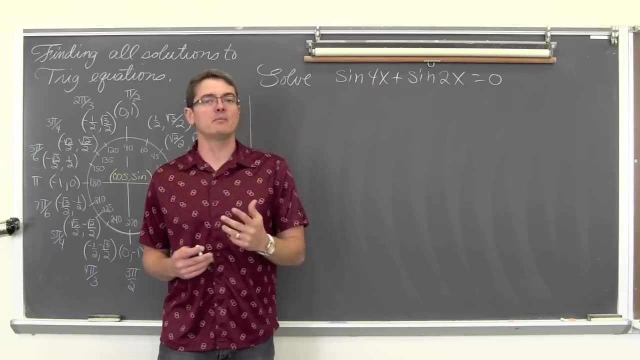 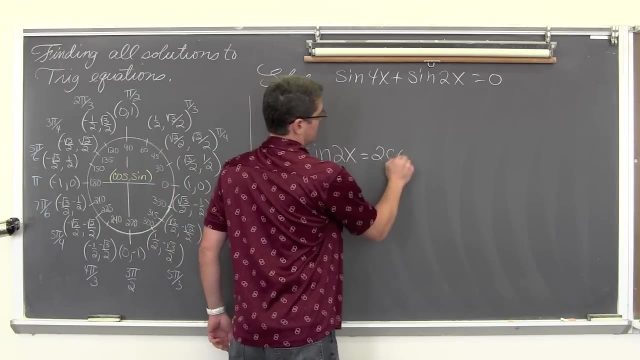 and those two variables factor apart. So we are going to take a double angle identity and that will allow us to reduce this angle measure of 4x and bring it down to a measure of angle of 2x. We are going to use the identity of the sine of 2x is equal to 2 cosine x- sine. 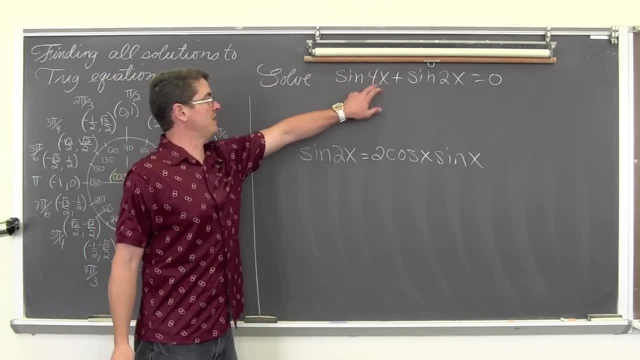 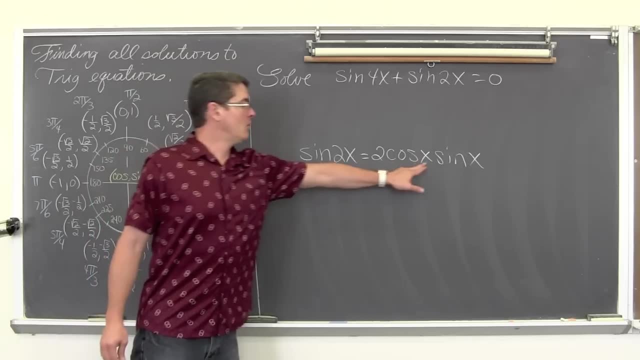 of 1x, But of course this is not a 2x, It is 4x. It doesn't really matter that this is 1's and this is 2's. This angle measure is double what we have on the other side of. 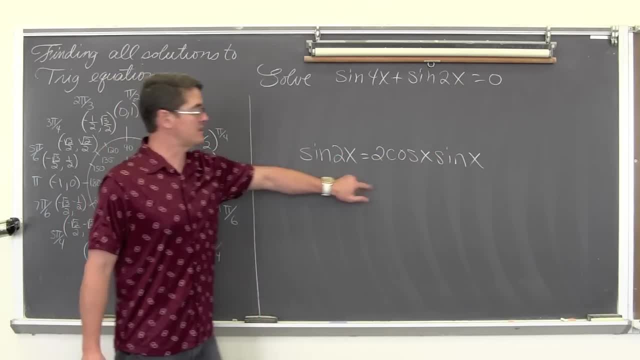 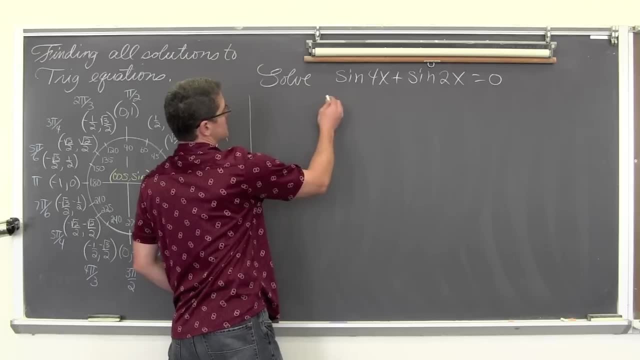 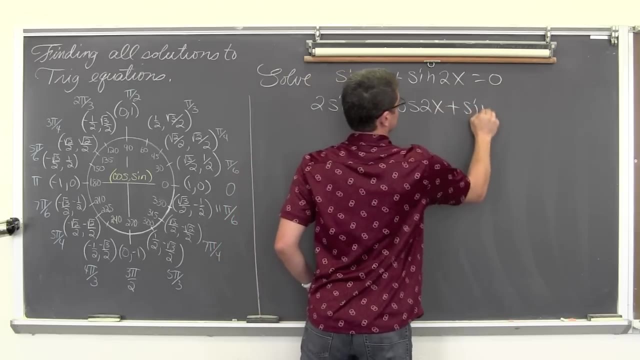 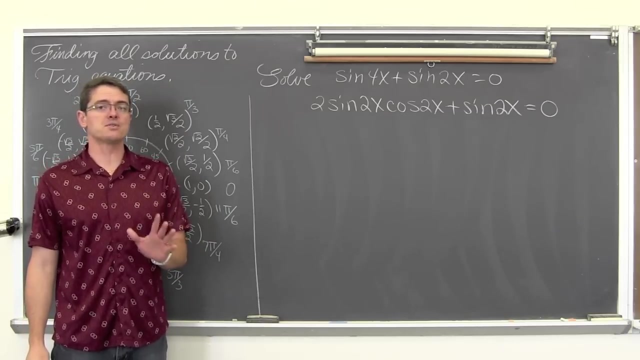 the identity. So this is the identity I am going to use, except there is going to be a 4x here, So these will be 2x's. So this identity substitution, We will get all of our angle measurements to be the same size. So we are getting closer. 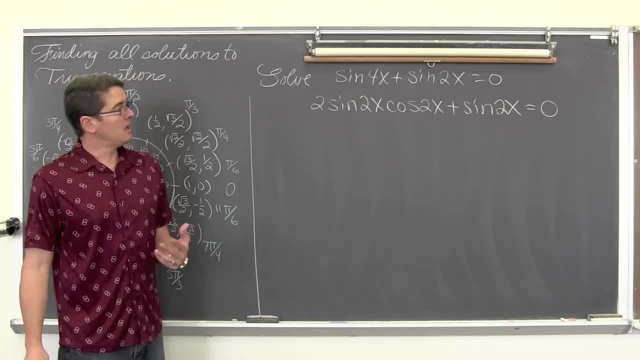 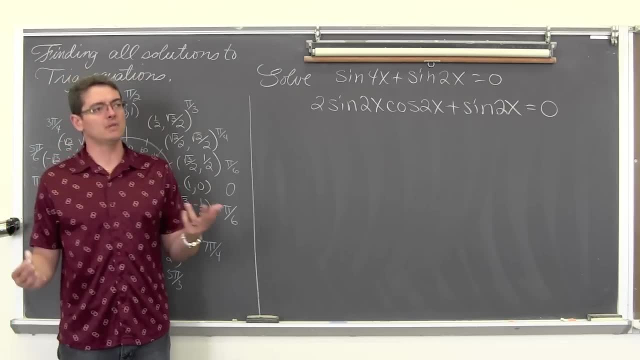 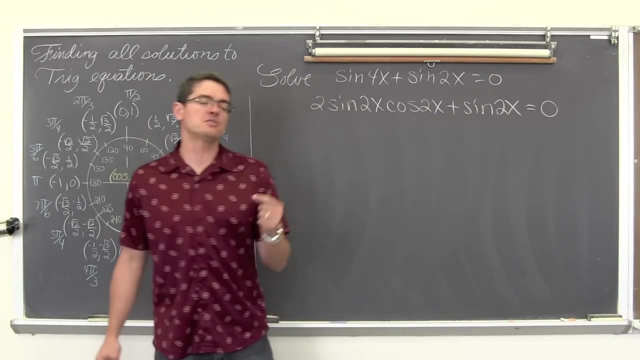 to getting ready to solve this. But now we have two different trig functions. We have sine and cosine, So still we have an issue here with the two variables basically in the same equation. That could be a problem, except both of these terms have a sine of 2x, So 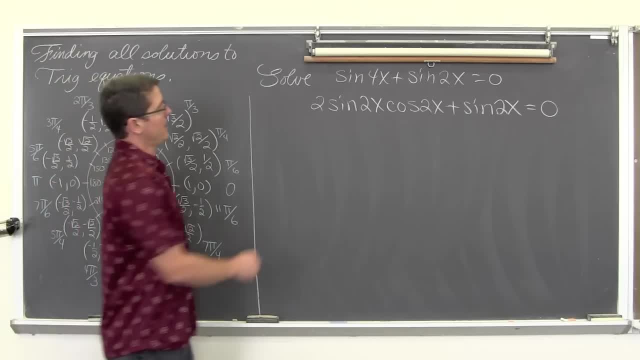 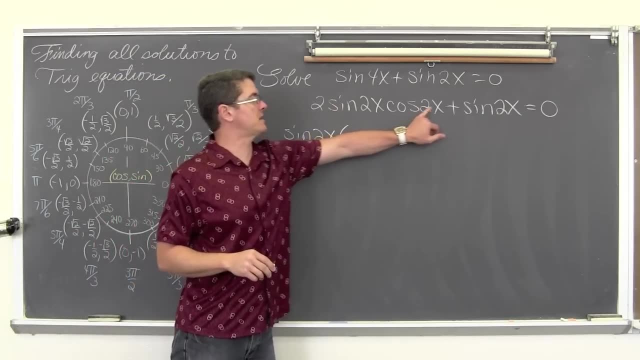 we can factor that out. We can undistribute that sine of 2x and get a sine of 2x. So sine of 2x times the sine, the 2. sine of 2x, cosine of 2x, take out the sine. 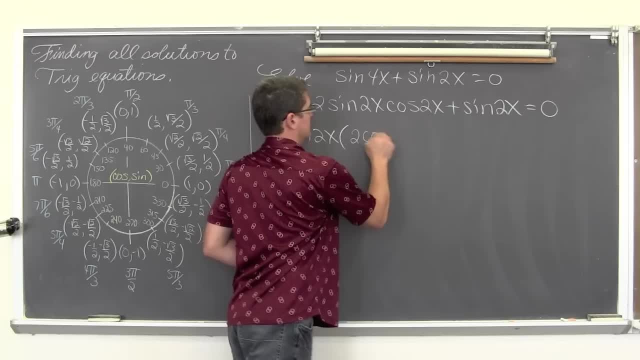 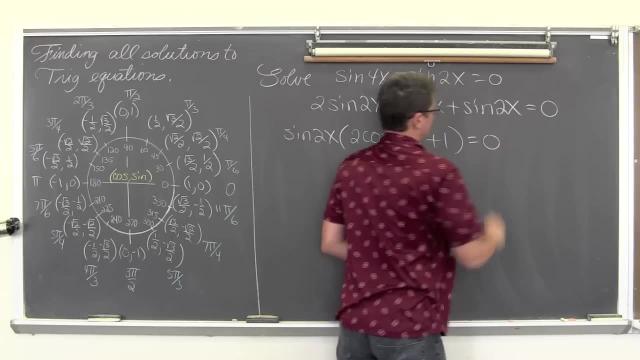 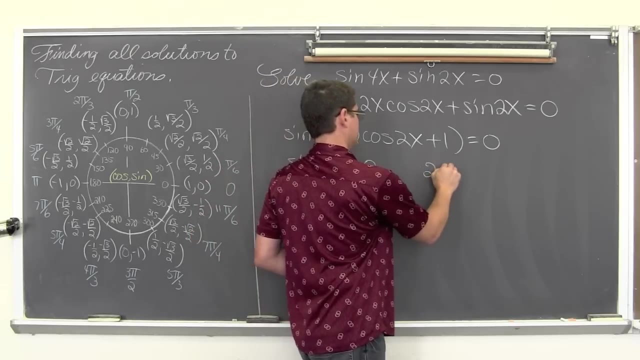 of 2x and we get 2 cosine of 2x. Sine of 2x divided by sine of 2x, of course, is 1.. We have it factored and set each one equal to zero. Get each trig function alone. I am going to 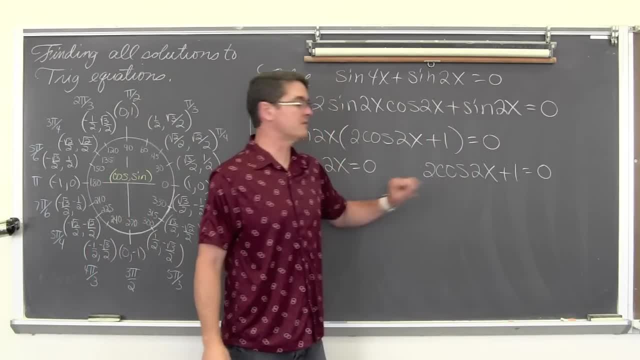 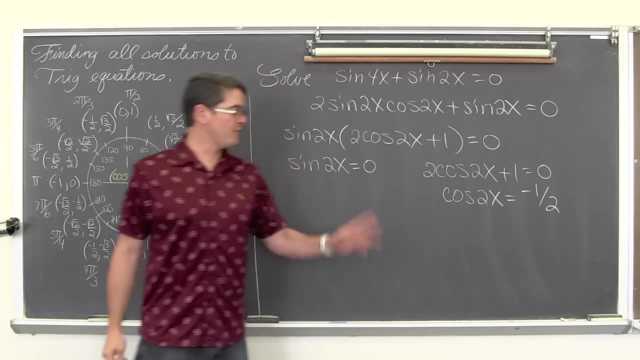 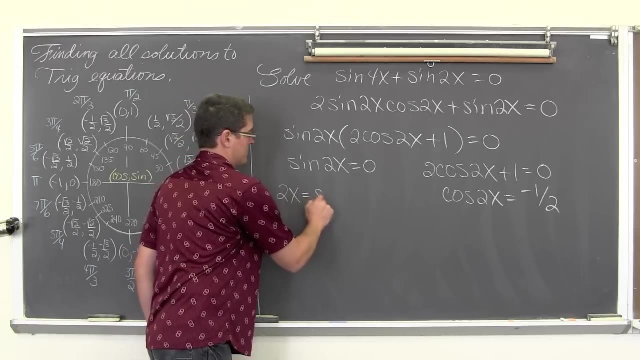 subtract by 1 and divide by 2.. So we get cosine of 2x equals negative 1, half. We are going to get those trig functions away from those angle measures by doing the inverse trig functions. So 2x is equal to the inverse sine of zero And 2x is equal to the inverse 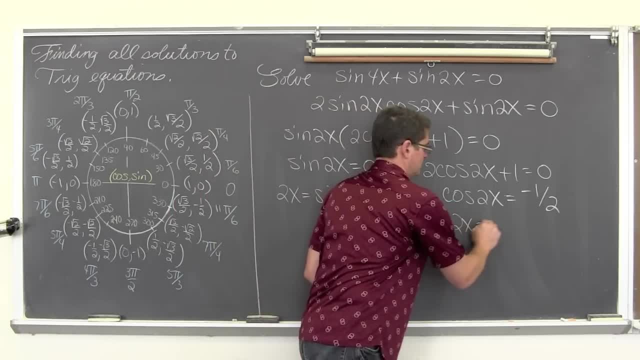 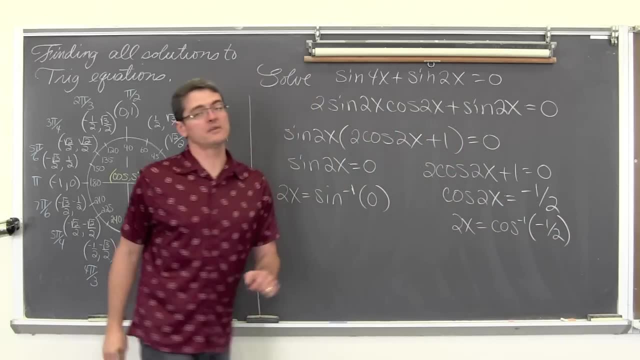 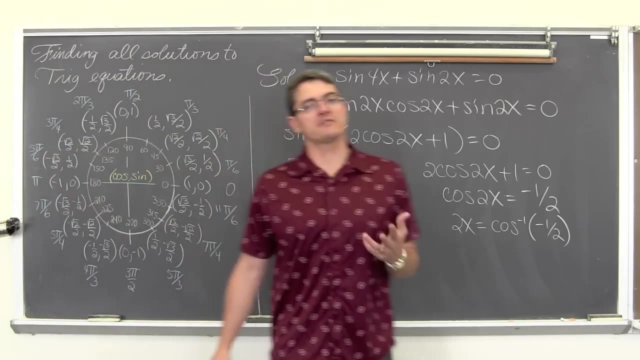 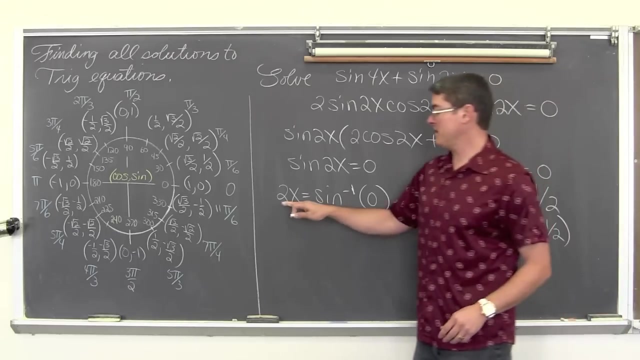 sine of zero And 2x is equal to the inverse sine of zero, And 2x is equal to the inverse cosine of negative 1 half. Now if we were only concerned about getting our values of x between 0 and 2pi, or 0 to 360- if you are doing degrees, then I would need to go around. 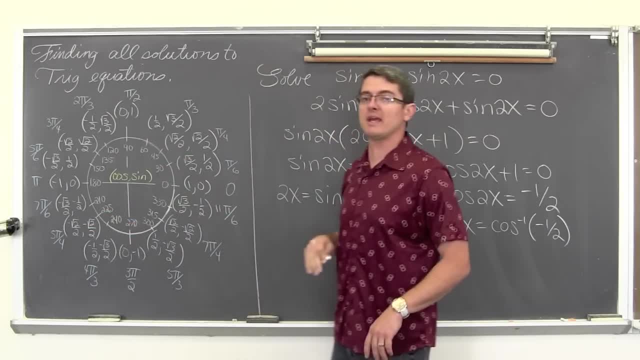 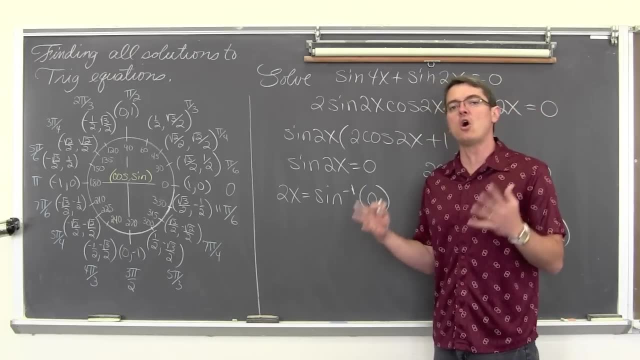 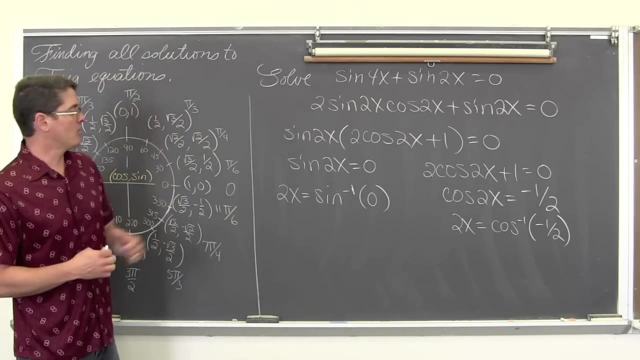 the unit circle twice and collect all of the possible answers so that I could divide them by 2 and get all possible solutions between 0 and 2pi. But we are looking for all of the solutions, Not just ones within a restricted range, So we are going to not worry about going around. 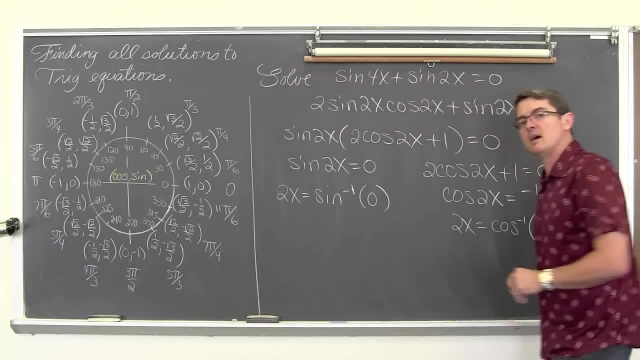 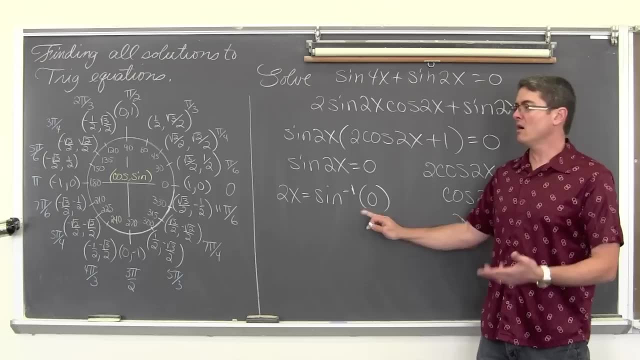 this unit circle twice. I am just going to do it once to find the angles I need And then add some little expressions there at the end to show that I want all possible solutions. Inverse sine of zero: where on this unit circle is the sine value equal to zero? Where the 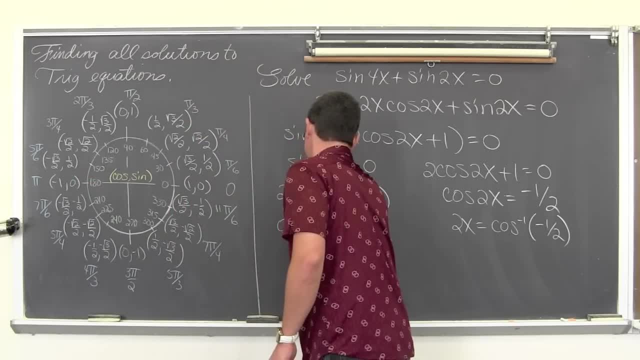 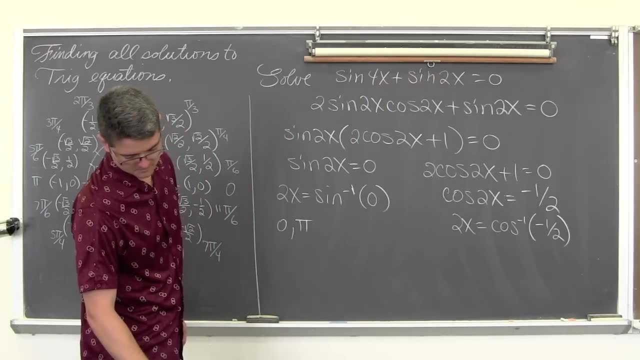 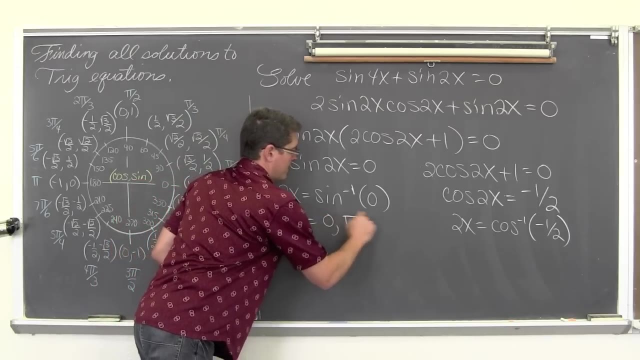 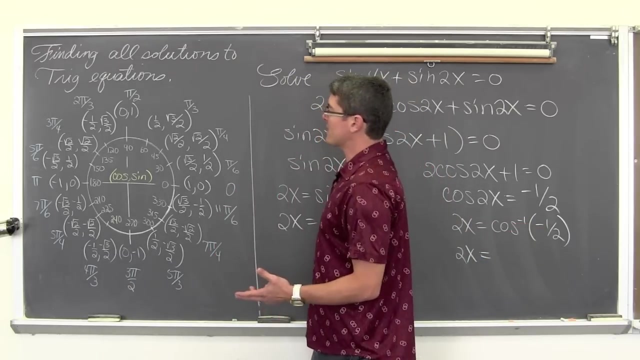 y is zero At zero and pi, And over here we have got. Oh, excuse me, I knew I forgot something: 2x equals zero and pi, And now we have: 2x is equal to inverse cosine of negative 1 half. Where is my cosine? Negative 1 half- Where? 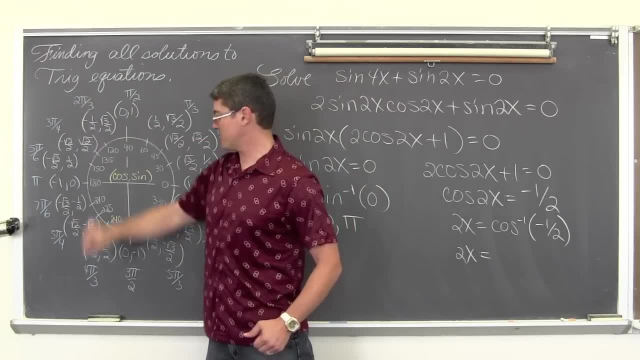 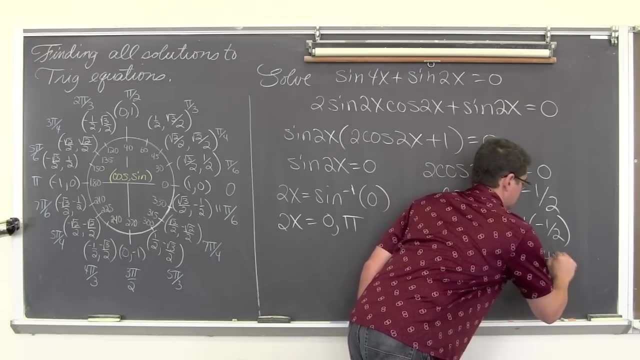 is the x values negative 1 half At 2pi over 3 and 4pi over 3.. Ok, We are just going to do that, Ok, Ok, Ok, Ok, Ok, Ok, We are solving for x and we are going to divide everything by 2.. So, dividing both sides by 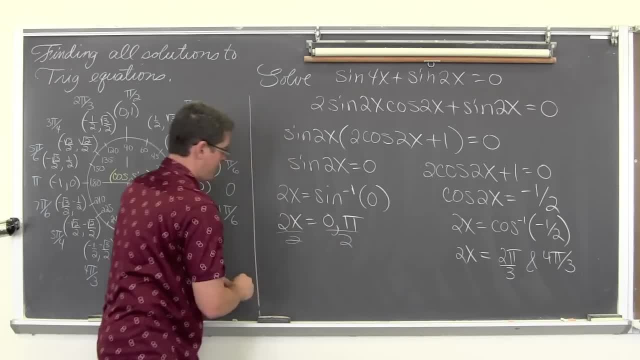 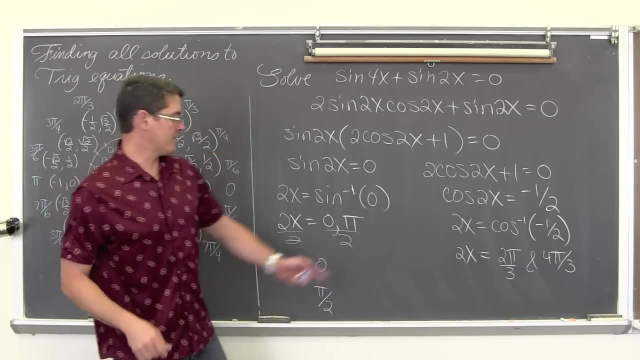 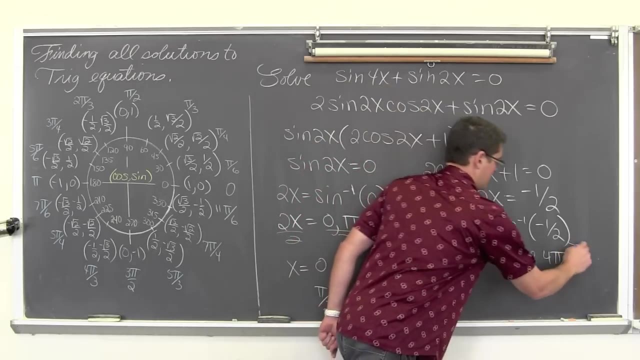 2. We have: x is equal to zero and pi over 2. Dividing everything by 2 over here, or because we have fractions, we are multiplying everything by 1 half, We get 2 times a half is just simply x. 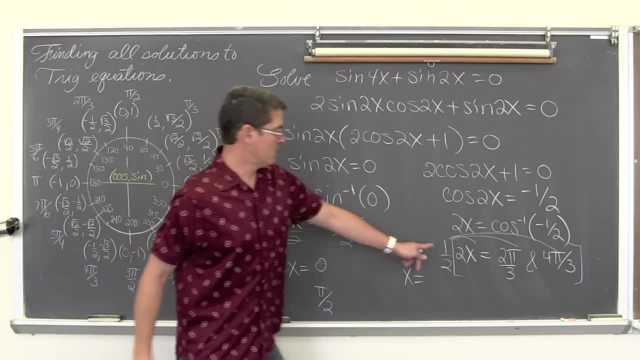 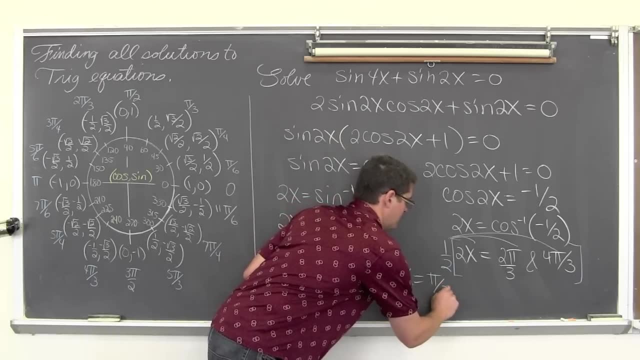 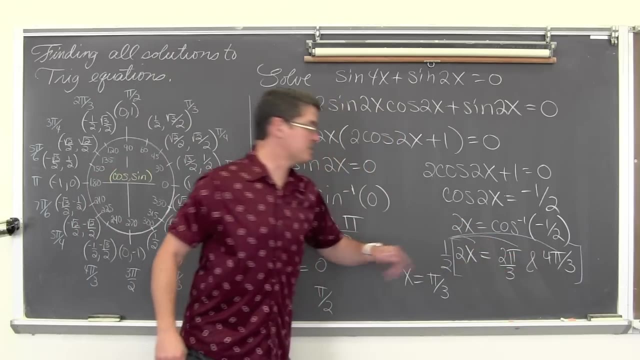 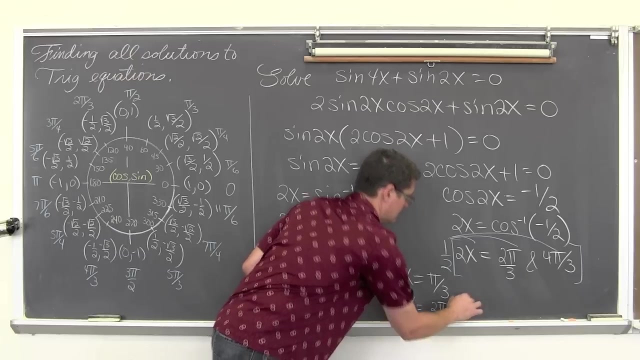 Ok, Then 1 half times 2 thirds: The 2's are going to cancel out, giving me pi over 3.. I am running out of room here. 1 half times 4 over 3.. 4 divided by 2 is equal to 2. So we have x equals. 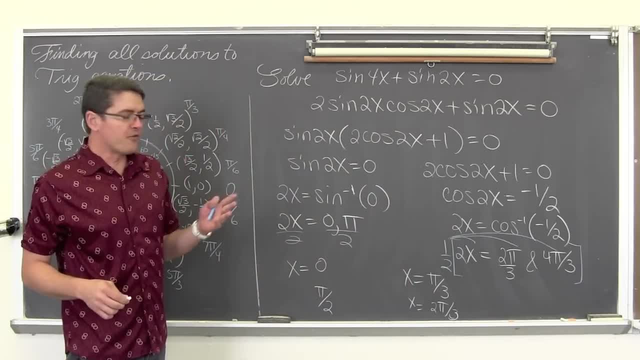 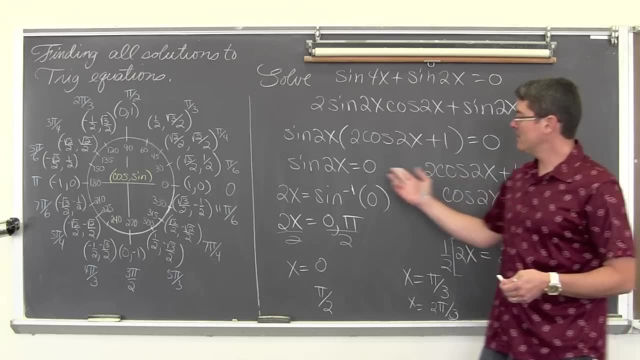 There we go: 2 pi over 3.. A little sloppy. there We have our four solutions that we need. But I don't want four solutions, I want all possible solutions. So let's think back to the previous example. We have a b value of 2. We have a sine function and we 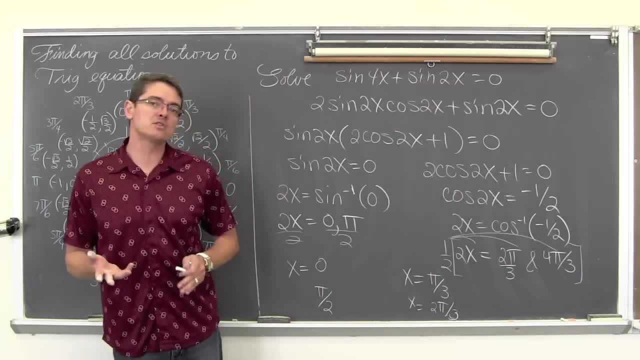 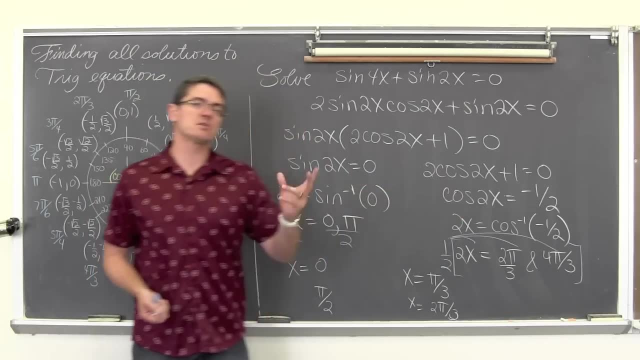 have a cosine function. The period of both of those strict functions is 2pi, So the period of 2pi divided by b. So each of these functions, because they are a double angle, when you were to go to graph them they would oscillate to do a full period within a distance, a horizontal. 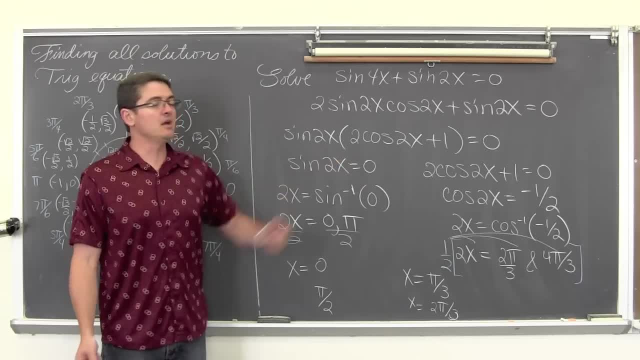 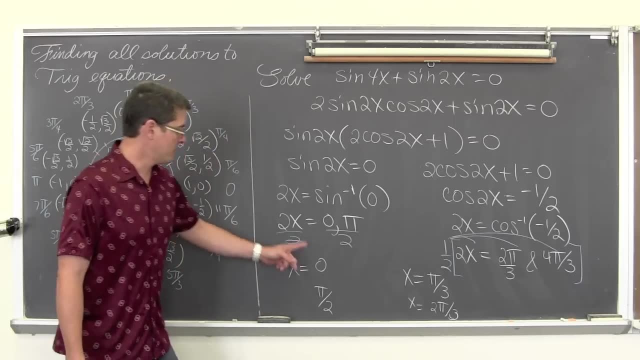 distance of pi. So, unlike the previous example, I am running out of time, So I am going to go back to the previous example. Here we only have a period of pi. To express that you want all possible solutions, you are going to go to each one of these and add in that it is. 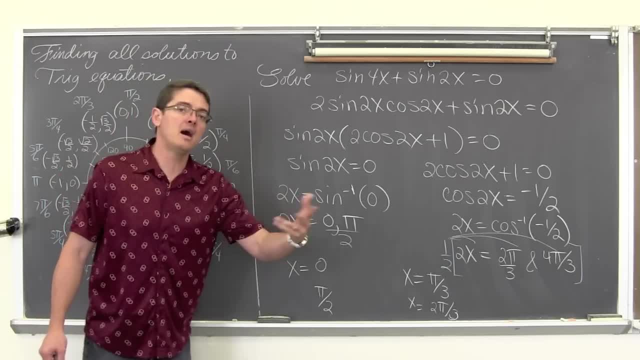 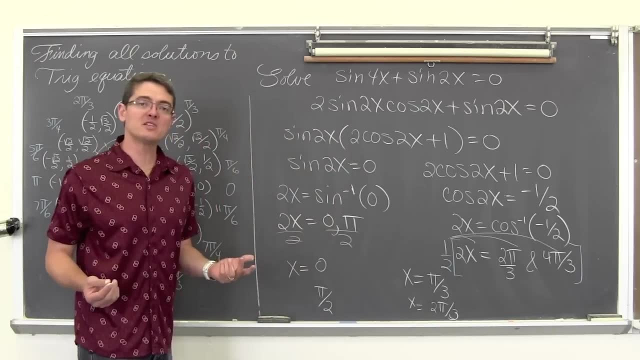 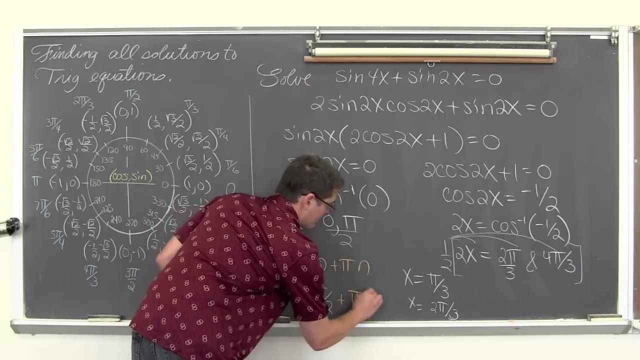 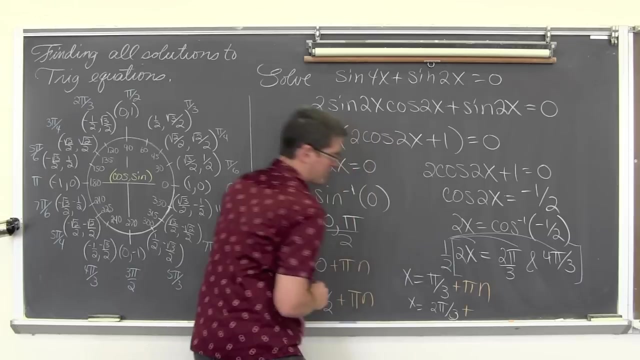 going to be this answer plus the period pi n, again where n is an integer. When you are done with that, you will have listed all your possible solutions. So 0 plus pi times n Pi over 2 plus pi, times n pi over 3 plus pi n, and 2pi over 3 plus pi n. And there we are done, We have answered. 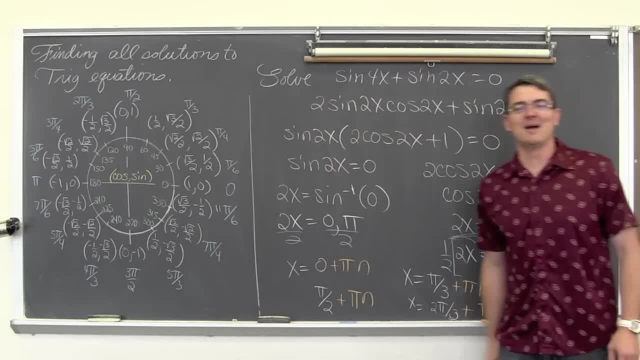 or given all possible solutions to our last example. I am Mr Tarrou BAM. Go do your homework. 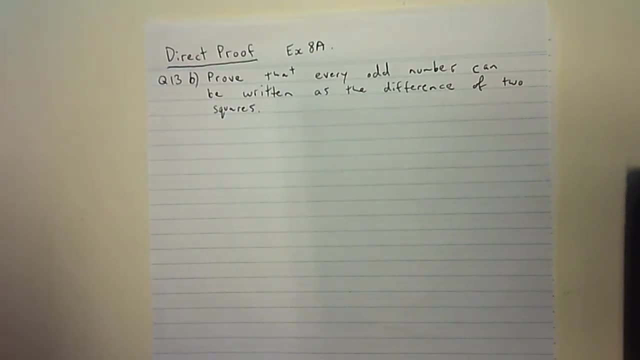 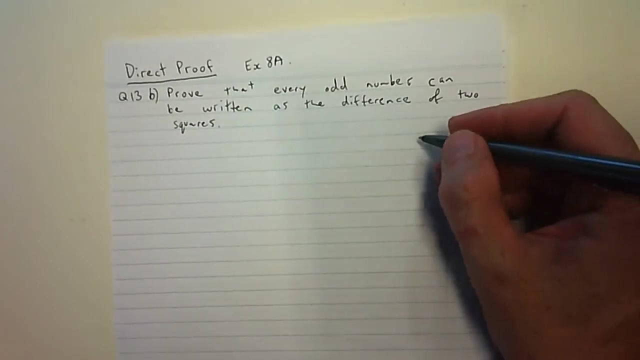 Okay, so I'm just going to do this to prove that every odd number can be written as a difference of two squares. Now we should probably recognise from the previous question if I was to get two squared and I take away one squared from it. 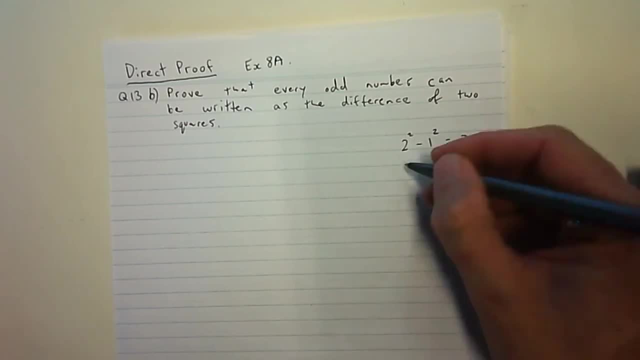 let's work that out. so that's four: take away one gives us three, And if I do three squared, take away two squared, I end up with nine. take four, which is five, Keep going on this four squared. 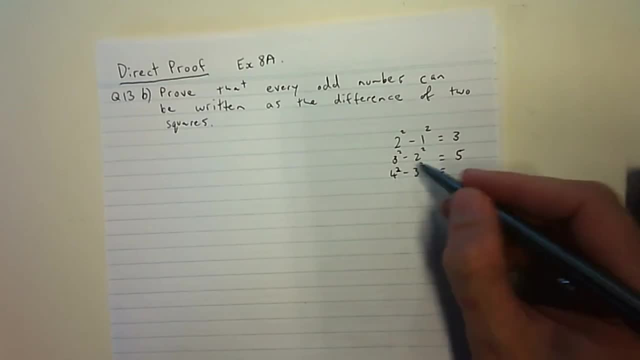 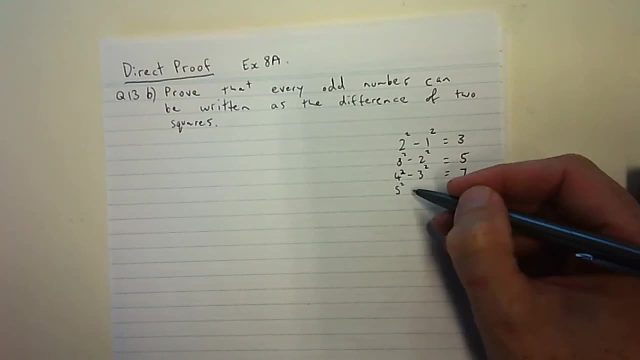 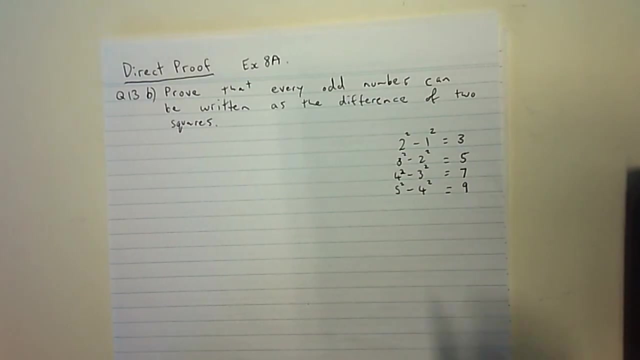 Take away three squared and we end up with seven. So sixteen take away nine is seven. And if I go five squared, take away four squared, okay, we end up with nine. Now, from this pattern, you can start to see. you can see what's occurring. alright. 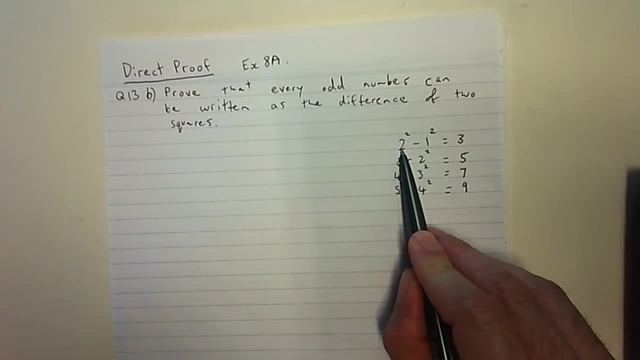 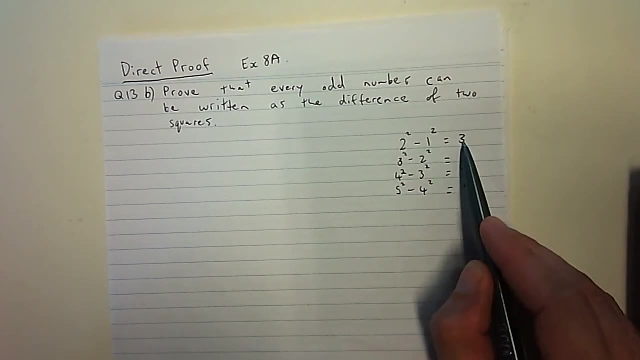 If I have a number and one squared and if I have one less than that squared and I take away, If I take them away from each other, it's the same as two plus one gives me three. Three plus two gives me five. 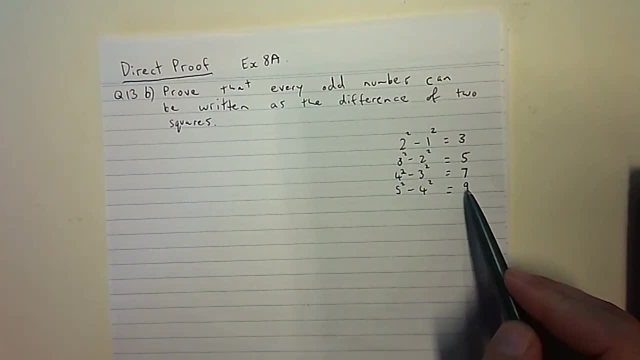 Four plus three gives me seven. Five plus four gives me nine. So we're seeing this pattern occurring, but we haven't proved it for every single case. We've only proved it for a couple of these cases. Okay, so we need to look at a way of proving it for every single case. 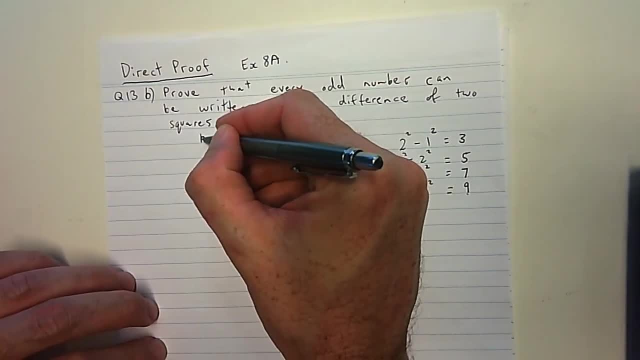 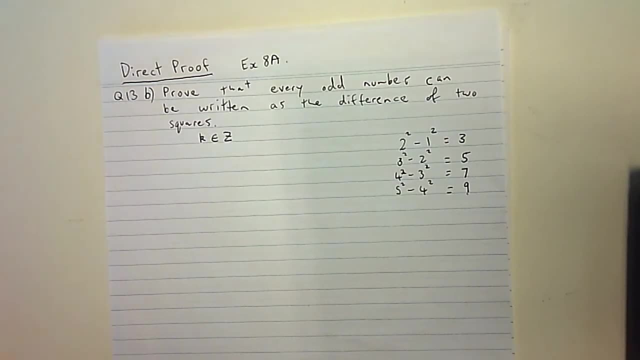 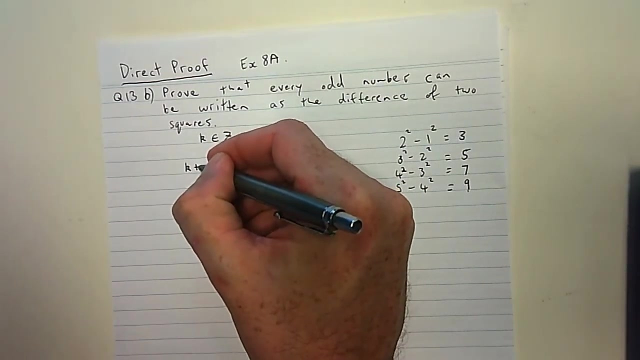 Alright, now start off by saying that k is an element of z. Okay, it's any integer. Okay, Any integer that you can think of. alright, And with this situation I want to be saying: well, if I have an integer plus one.